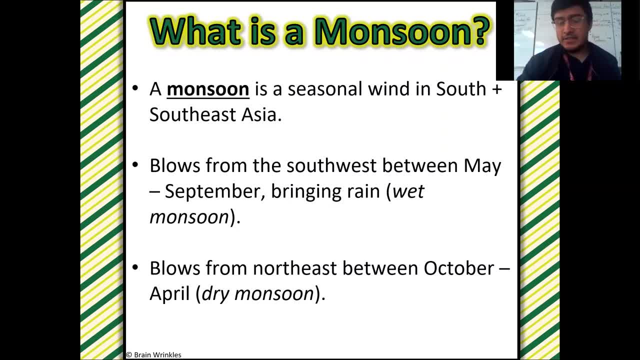 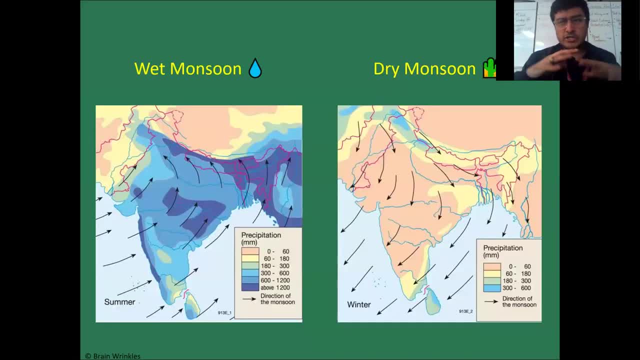 It is not a storm. Okay, a monsoon again. is that seasonal wind that tends to bring with it a lot of storms and rainfall? Okay, almost like a culmination or cause of storms in a lot of areas of South Asia. Okay, 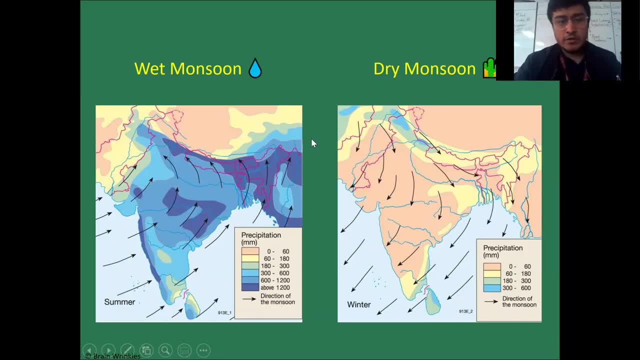 so here on these two maps they're going to show us the wet monsoon in South Asia. that tends to happen around the months of the summer months. The actual monsoon winds here are visualized with the arrows, And then the other month, so the winter months. 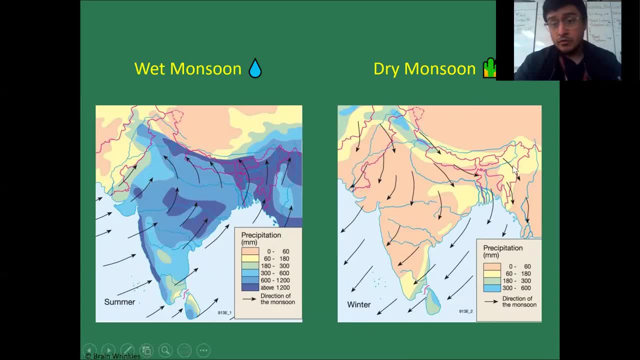 in the beginning of the spring months are going to be the dry monsoon winds coming from the Northeast. Okay so wet monsoon winds coming in from the Southwest here during the summer And then during the winter and spring months it's going to come in from or the monsoon the dry. 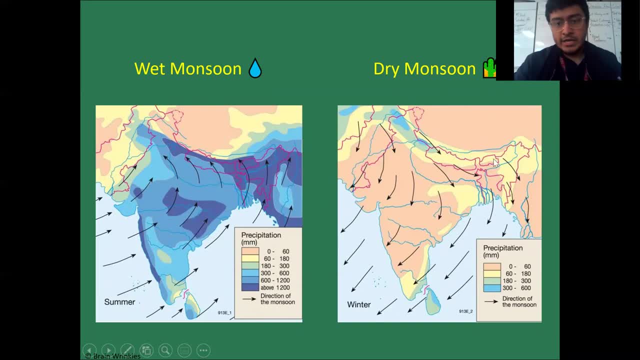 monsoon winds are going to come in from the Northeast here. Okay, and again, all this is going to be South Asia, right, India here being the biggest country in South Asia. We're going to talk a lot about that in the next couple of weeks, So thank you so much for watching. I'll see you. 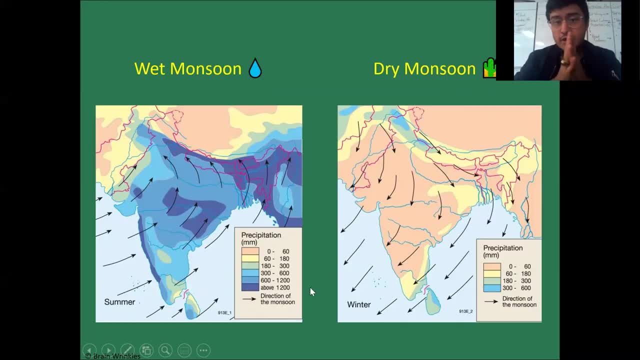 in the following lessons. Okay, so some questions that we're going to go ahead and just take a moment to either answer by yourself at home, virtually, or in class. Just some map reading questions are going to help us practice with actually reading different types of maps. this: 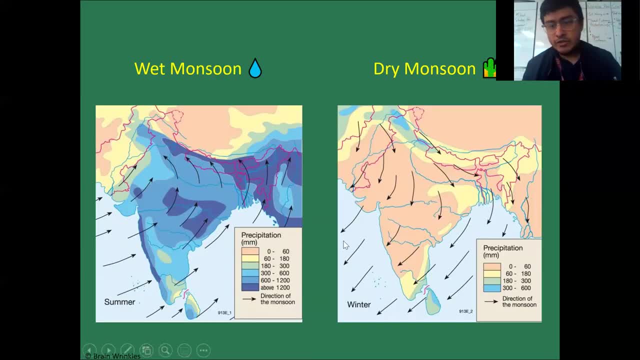 one being a precipitation or a rainfall map. Okay, you see all the pretty colors here in both maps and they're going to be indicative of the amount of rainfall in millimeters for each region here. Okay, so, like the area around the middle part of 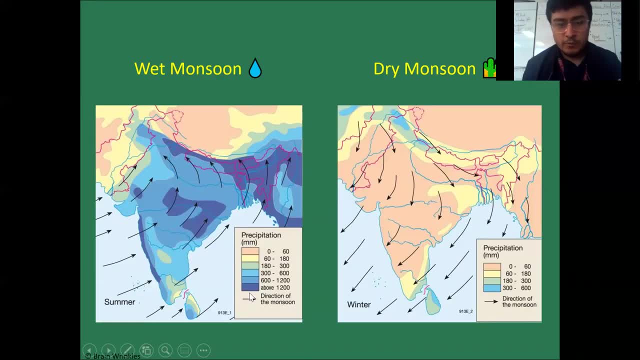 India during the wet monsoon is going to have quite a bit of rainfall, around 1200 to 600, even going a little bit lower up until like 300 to 600 in those parts of India. Okay, so you really just have to look at the colors here and see where they correlate with the colors here on the map legend. 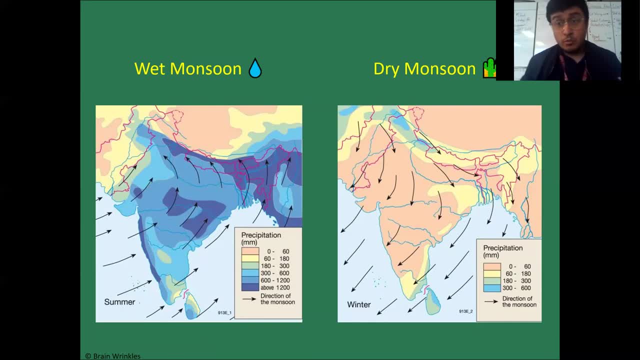 to see what the precipitation level is. Okay, so first question to go ahead and answer, either by yourself or in class. First one is: how much rainfall does the country of Bhutan get during the wet monsoon? Okay, so the country Bhutan is going to be this little one right here. 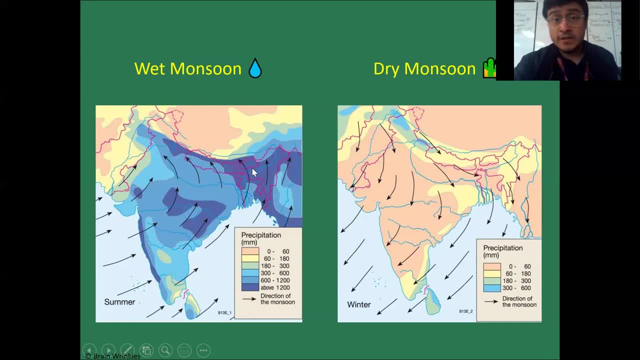 So, using the map legend and you know just your map reading skills, how much rainfall does this country of Bhutan here in South Asia? how much does it get during the wet monsoon? Okay, so hopefully you all had a moment to pause and think of that over. 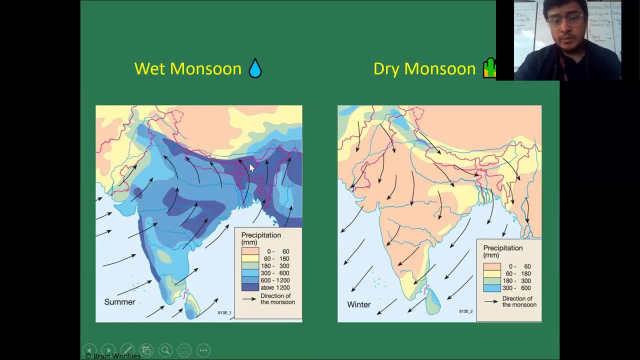 So the answer to that, how much rainfall does Bhutan get during the wet monsoon? is going to be quite a lot. so above 1200, so over 1,200 millimeters of rainfall during the wet monsoon. Okay. so second question: how much rainfall occurs in the southwestern part of Sri Lanka? So Sri 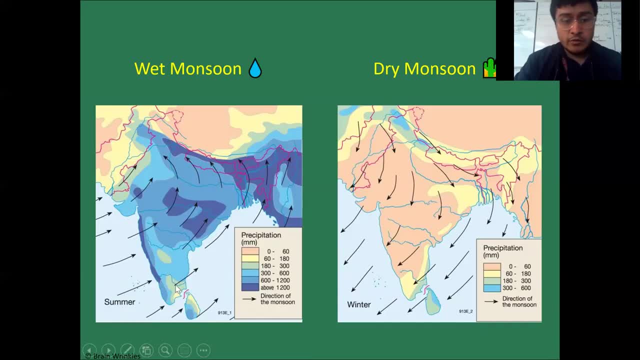 Lanka is going to be this little island area here off of the coast of India, the southern coast of India. so that's Sri Lanka here. Okay, so the question again is: how much rainfall during the wet monsoon season? how much rainfall does the country of Bhutan get during the wet monsoon? 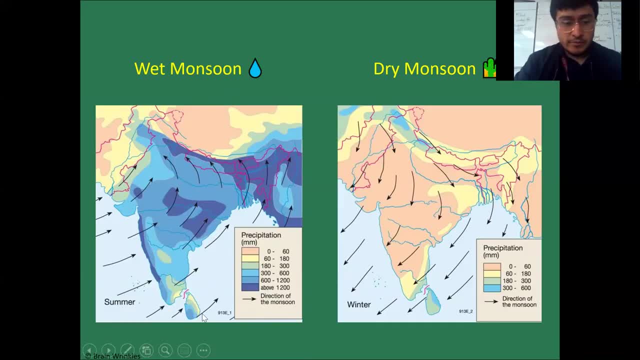 of sri lanka, get in the southwestern part of it. okay, in the southwestern part of sri lanka, how much rainfall does it get? all right, and after discussion or thinking about that, and if you came up with 600 to 1200 millimeters of rainfall, then you'd be correct, so you can go ahead and pay yourself. 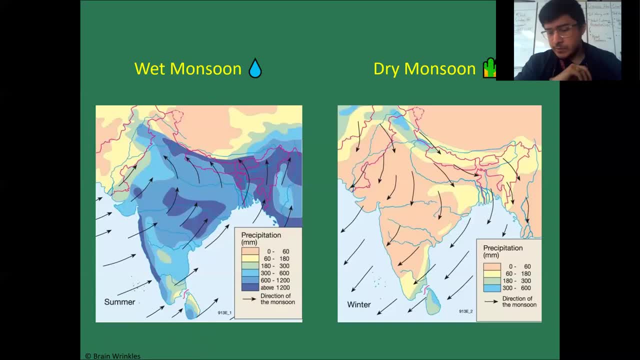 on the back for that one. uh, so the third and the final question: annually, which means year round, so you have to be looking at both maps here. so, year round, which side of india's coast, west or east, gets more rainfall? okay, so remember, india is this giant country here in both maps. 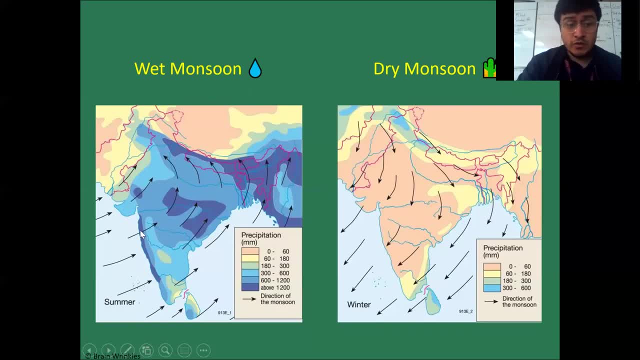 and the question again is: which side of india's coast- so the coast being all along here both sides- which side of india's coast gets more rainfall? is that going to be the western coast side or the eastern coast side, year round? okay, so you might have to do some little. 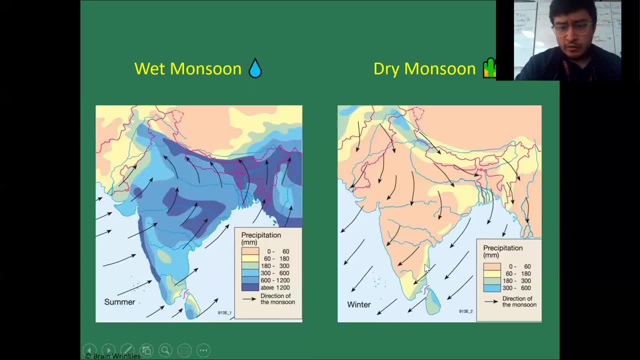 approximately mental math here with addition. So, year round, is it the west part of India's coast or the eastern part of India's coast that's going to get the most rainfall? What do you think year round? Okay, hopefully you get that some thought. And if you ended up coming up with the western 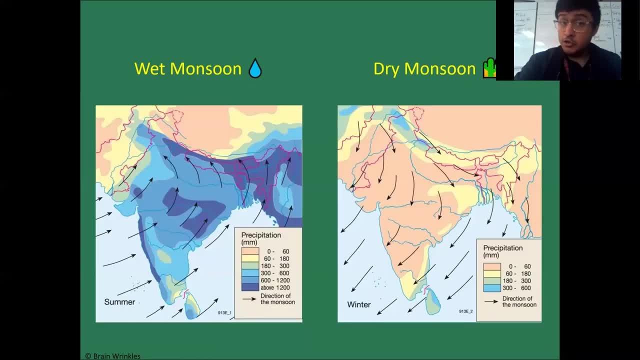 coastline for India getting more rainfall annually? you'd be correct, And the easy way to look at that is seeing here. there's a whole bunch of over 1200 millimeters of rainfall constantly around the areas of the western coast here in India, Whereas over here it's quite a. 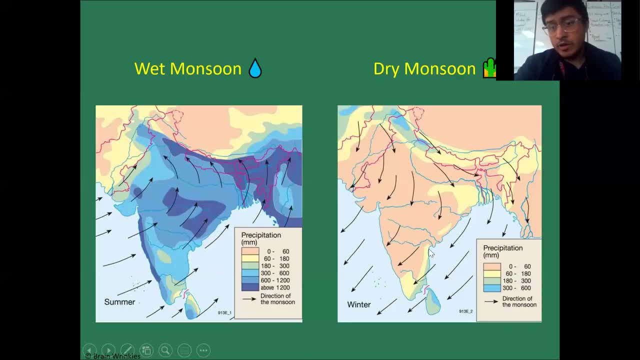 bit less And, honestly, it's the same for the most part on the other side as well, And there's just going to be a whole lot more rainfall. that occurs on the western part of India's coast, the west side, versus the eastern part of India's coast. Okay, so keep. 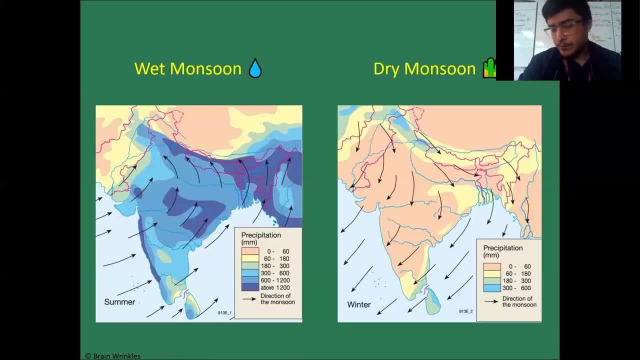 that in mind And hopefully sharpened up your map reading skills here with those few questions. Also, before we move on, just a question: Why? Okay, so kind of get into that critical thinking aspect. Why do you think the western part of India's coastline gets more rainfall yearly or annually? 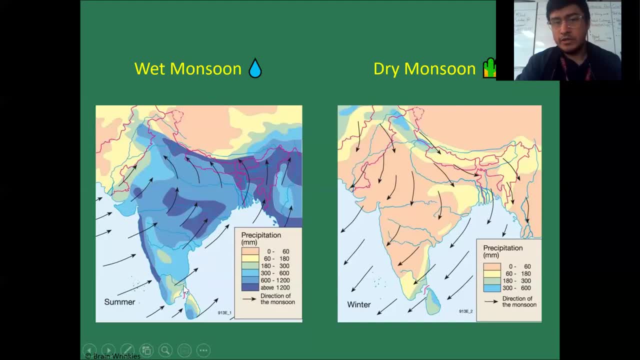 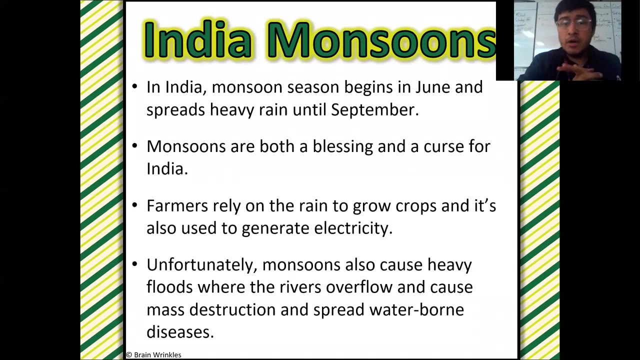 compared to its eastern part or the eastern coastline here in India. Okay, so just a little food for thought there. Okay, Moving on, we're talking about specifically India's monsoons, kind of like what we're talking about with the map. So in India, monsoon season does begin in June and spreads heavy rain. 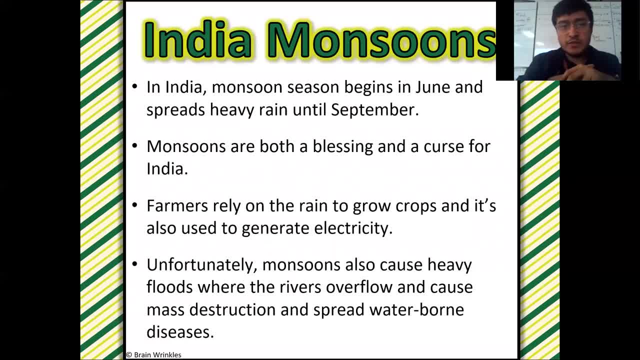 up until the month of September, So pretty much during the summer months, it's going to be a lot of heavy rainfall in India. Now, monsoons are both a blessing and a curse. That means there's a lot of positives and negatives for India and, honestly, a lot of. 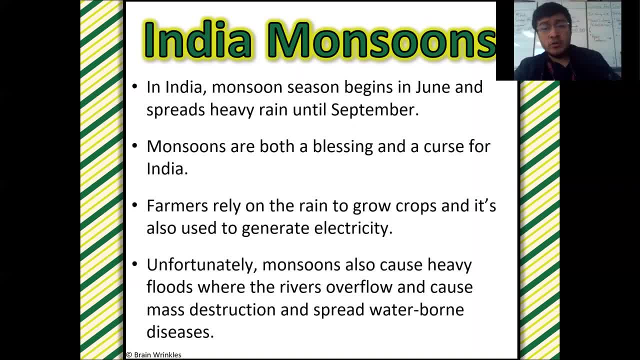 the other South Asian countries as well. So farmers rely on the rain to grow crops, and it's also used to generate electricity. So those are two good positives that come from monsoon rains in India. Okay, so lots of rainfall means lots of water for the crops. 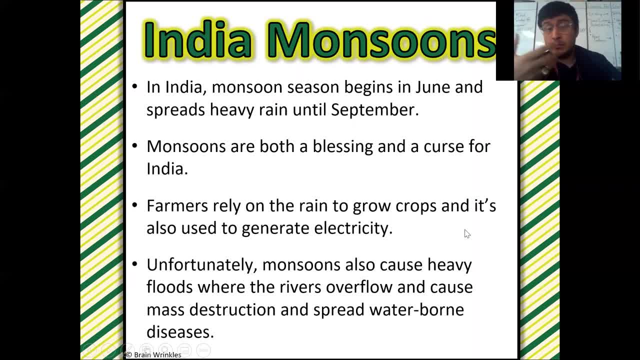 to grow, and lots of rainfall also means that people are able to use water for damming it up, and they're able to constantly filter that water and kind of have it flow and generate electricity. So those are positives. Now here, in this last bullet point, it's going: 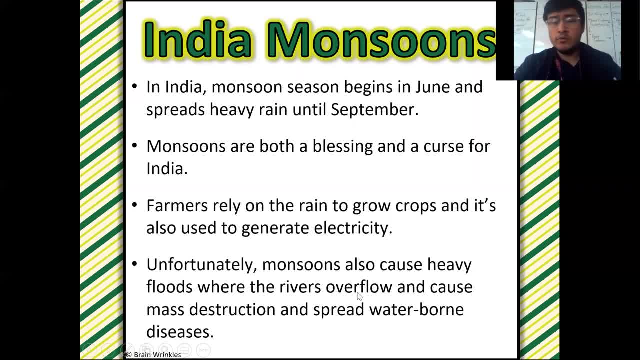 to be talking about the negatives. So unfortunately, monsoons also cause heavy floods where the rivers overflow and cause mass destruction and spread of waterborne diseases. Okay, so there tends to be a lot of negatives that come from monsoon winds and rainfall mainly. 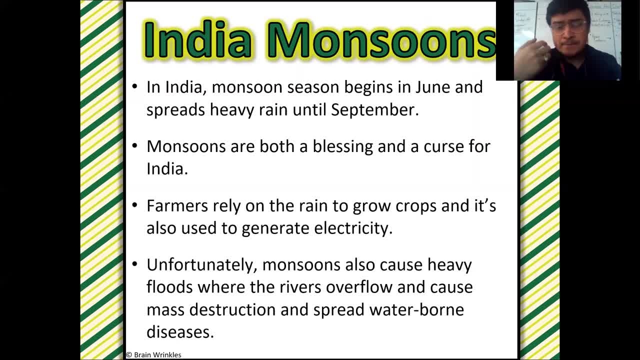 being the risk of heavy flooding. Okay, so you can just imagine the dangers of constant flooding waters, especially when you start getting into the aspects of waterborne diseases like cholera, where if there's a river that is very dirty and it has cholera in it, well, 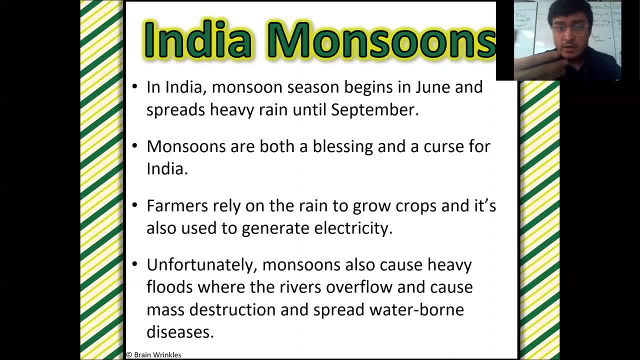 if it overflows, and it's flowing into the town, destroying all the buildings, and people are getting basically having to swim in it And they're exposed to that disease, cholera, then they're going to end up, you know, contracting it. Okay, on top of the fact that the floodwaters are going to be ruining their houses, their 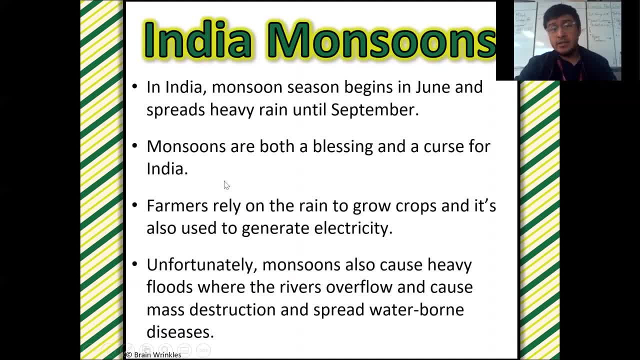 cars, their property, what have you? Okay? so again India. monsoons are honestly monsoons just in general in South Asia. They have their positives, their good things, and their negatives are very bad things. All right, Okay. so next few slides here are going to: 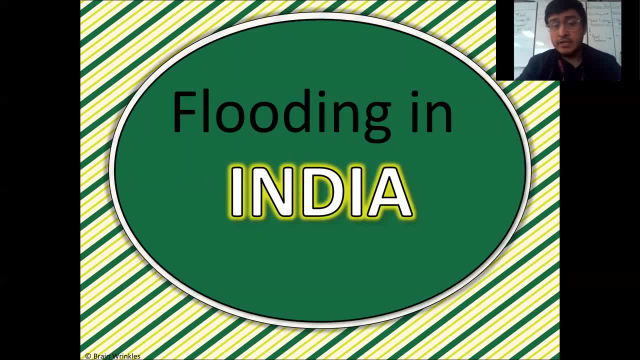 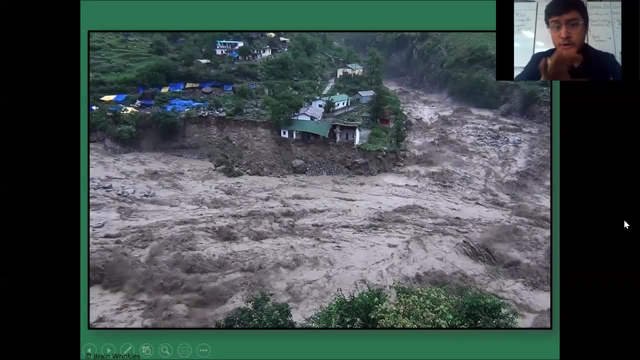 be getting into actual images of floods in India that have been caused by, you know, by those monsoon rains. Okay, so here I don't know exactly where India this is, but it is going to be in India. You'll see that a river. I want to assume that the river probably 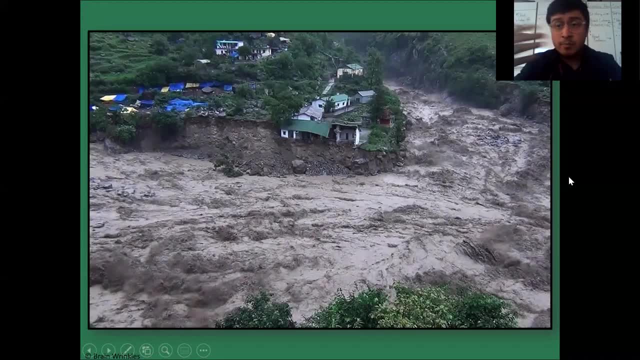 was like around this area here, but because the heavy rainfall that was brought about by the wet monsoon during the summer months most likely made the river overflow and it's just a complete disaster, for not just the earth and the ground, you know, picking up. 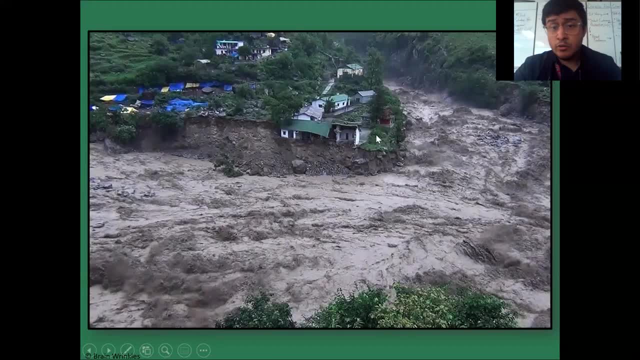 all that soil around it. So these houses that these Indian people had along that river line there, okay, it's just way too much water, way too much flooding, and it's taking away the foundation that is holding them, holding their houses, you know. on the ground, So a lot of damaged property. 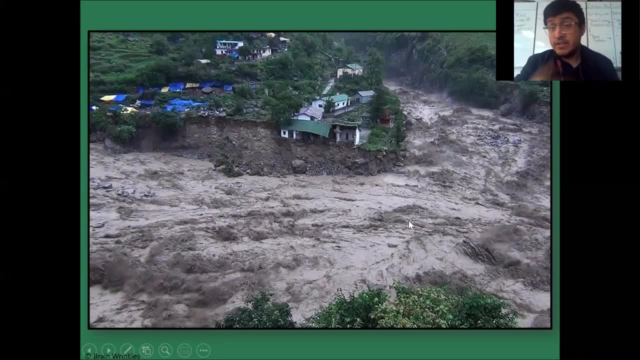 Okay, and again, you can even imagine that if there's diseased water in there, the floodwater or the flooding brought about by the monsoon rain is just going to, you know, worsen it and make it more likely that those people are going to contract that sickness in the 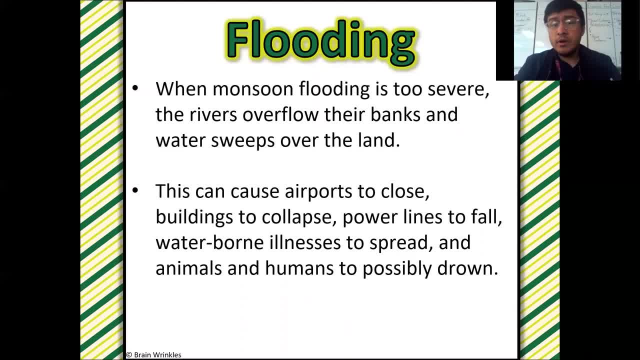 water, Okay, Okay, so flooding. So whenever the monsoon- flooding, as we just saw, is too severe, rivers are going to overflow their banks and water, just you know, constantly streams over the land. It's kind of like you're filling a water bottle too much. It's just going to overflow. 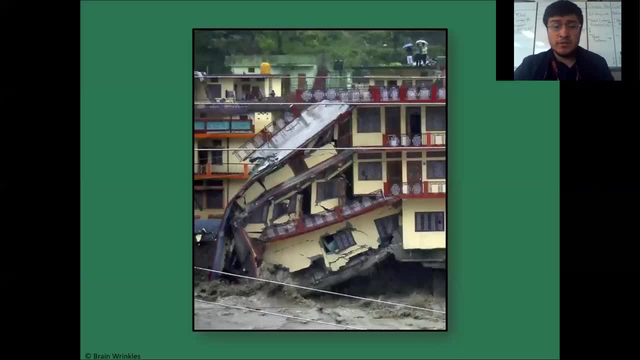 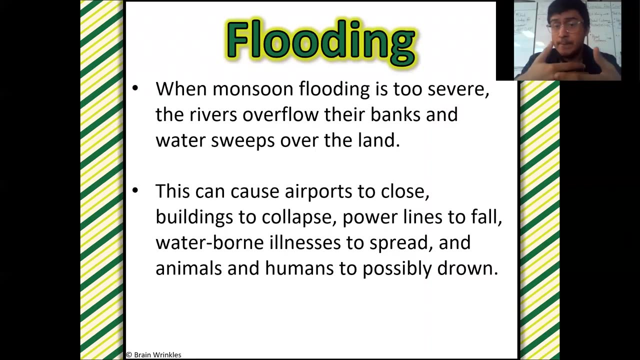 This can cause airports to close, buildings to collapse, power lines to fall, waterborne illnesses to spread and animals and humans to possibly drown. Okay, so just way more of those negatives are those bad consequences that come about from the monsoon rains flooding those rivers. 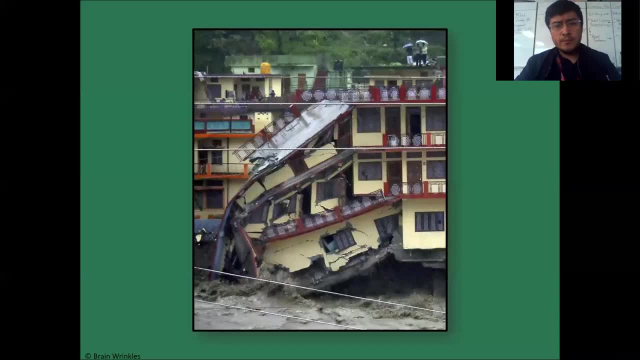 All right, so again, just another image here of an Indian building that is succumbing to the horrible effects of flooding caused by monsoon rains. Okay, so the floodwaters are taking away the foundation, they're taking away the dirt, the earth that is under the building. 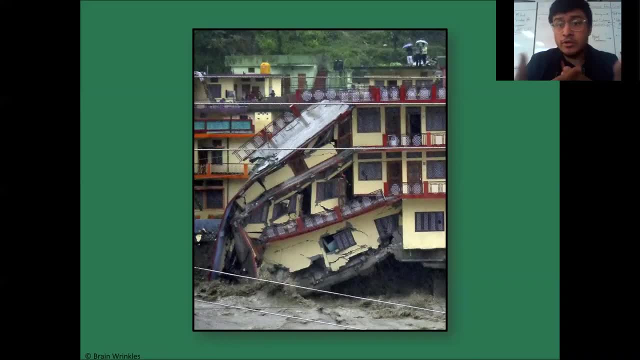 And then, obviously, if there's nothing for the building to be on, it's going to just crumble underneath its own weight. So there's very important for it to stay dry And in place. that way, the building is able to maintain its structure and it doesn't, you know, fall. 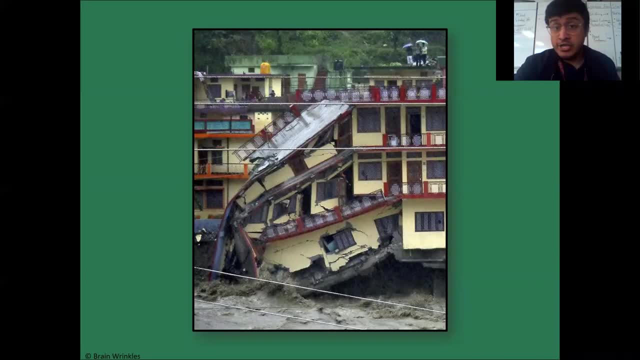 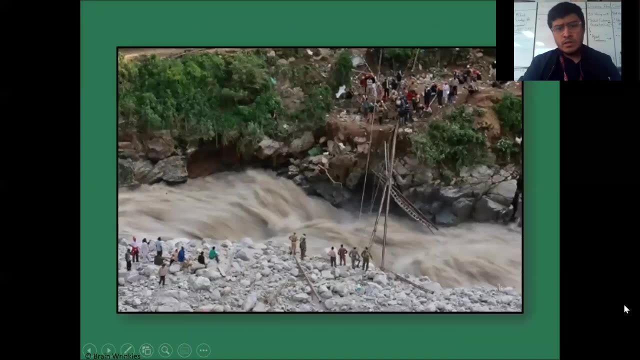 It's kind of like yanking the bottom Jenga block off of you know your Jenga tower, and then it's all going to fall down because it lacks that foundation like what we see here. So then, for this last slide, just again another pretty horrifying depiction of the dangers of the floodwaters. 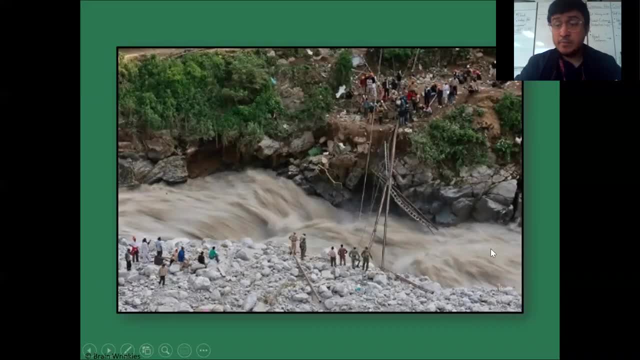 It's a still picture, but then you'll notice that the actual waters themselves in the picture are quite blurry, Okay, which means that they're going probably very fast. So it doesn't even matter if you're a good swimmer or not. 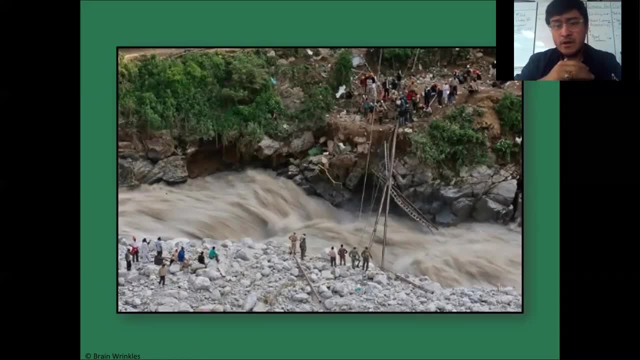 If you know how to swim waters that are going this quickly and to this degree, this volume, this amount of water there really isn't going to be a good chance that you're probably going to honestly survive this if you were to be swept up in these monsoon floodwaters. 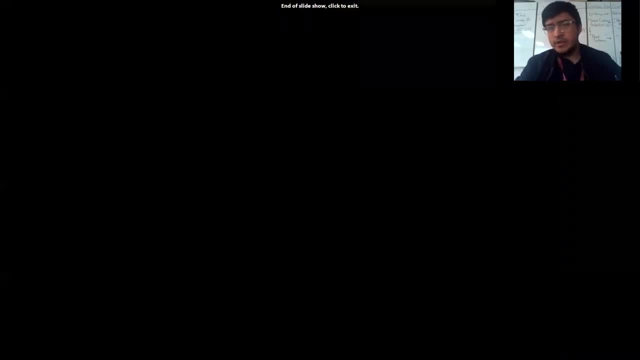 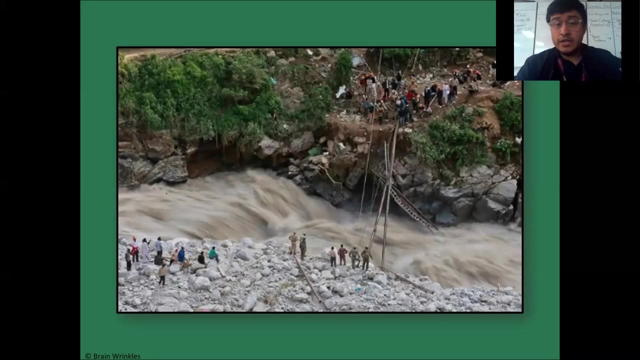 Okay, All right, so that is going to go ahead. Should be the last slide, Yep, So that's going to go ahead and wrap up our lesson, our very brief lesson, here over monsoons, And then we're going to move on to a few more questions. 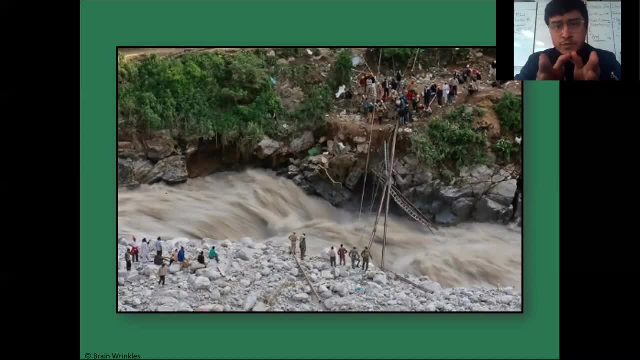 And we're going to talk a little bit more about what exactly the monsoon is and what it looks like in South Asia and just South Asia in general. So today's folder, there's going to be a couple of videos. The kind of very short videos are like one two minutes long.